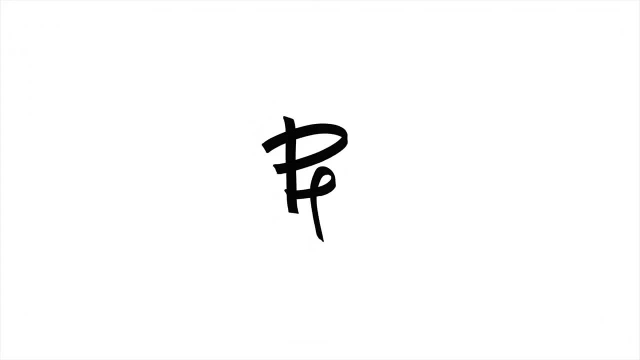 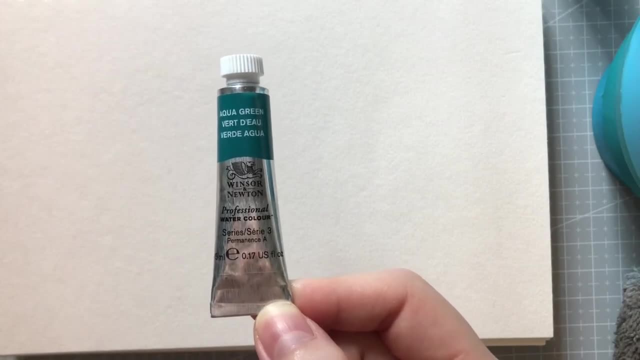 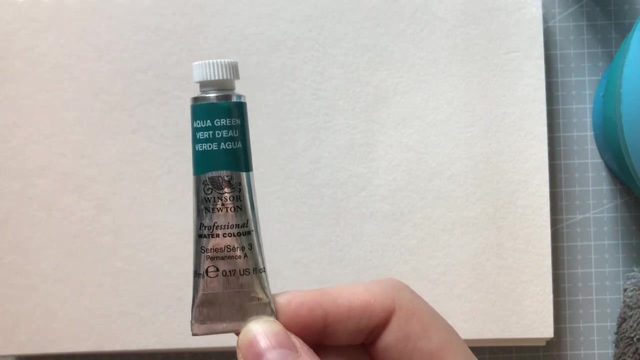 Hi everyone. So today we're going to be taking a look at Winsor & Newton's Aqua Green. The reason this is a standalone video just solely looking at Winsor & Newton's Aqua Green is because, you know, I like my turquoises. I love phthalo turquoise, pb16, and the first time I got to 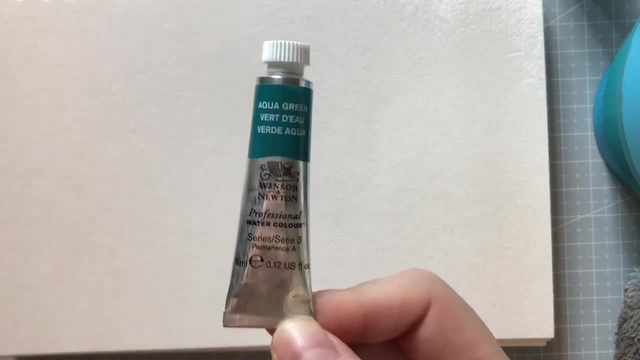 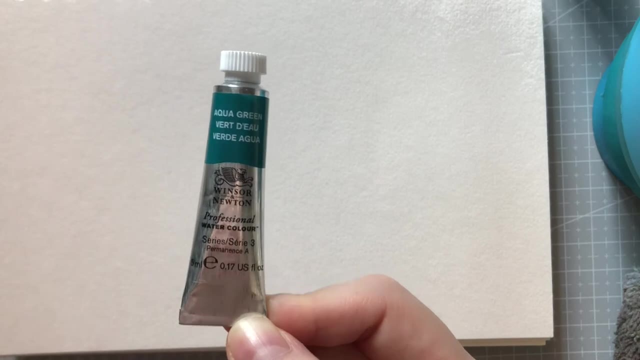 try. this Winsor & Newton's Aqua Green was when my watercolor fairy so kindly gifted me lots and lots of colors and one of those was a small pan of this Aqua Green and I just fell in love with it. It does lean a bit green, so I'll swatch it out for you and then, hopefully, 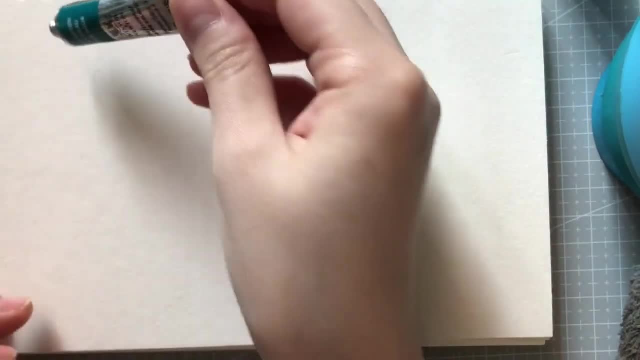 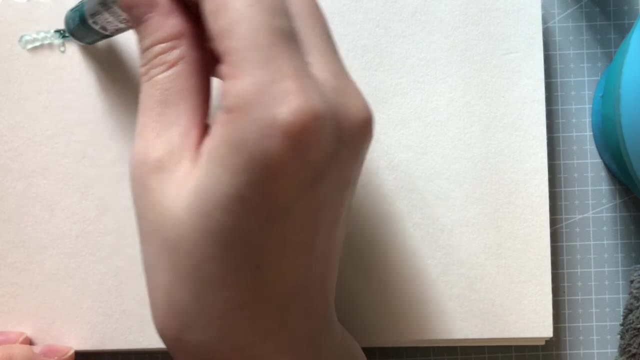 I can compare them to a few phthalo turquoise. A few phthalo turquoises. Oh no, has it separated already? You know what, we'll just go with it. So there's a lot of separation. so if you do, 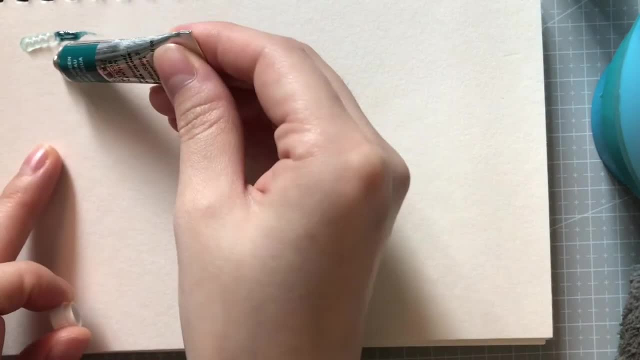 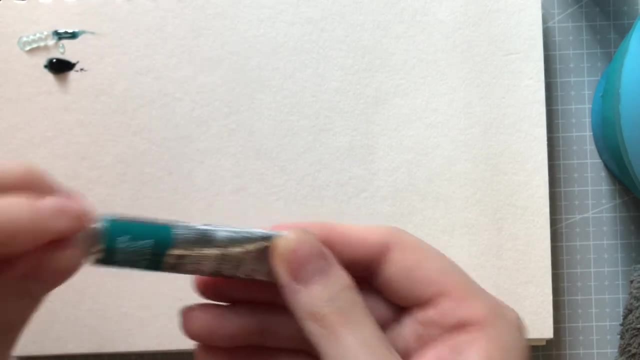 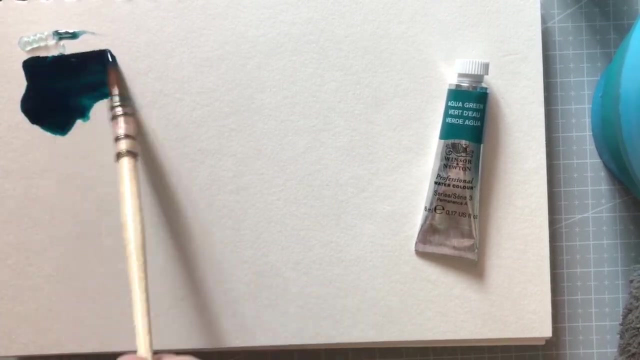 buy it, you're going to be able to see the difference. So I'm going to try this. Winsor & Newton's Aqua Green. Do beware. maybe you want to like stir your tube a bit, but you know what, for today I'm just going to go with it, All right, so let's take a look together. It's definitely a very 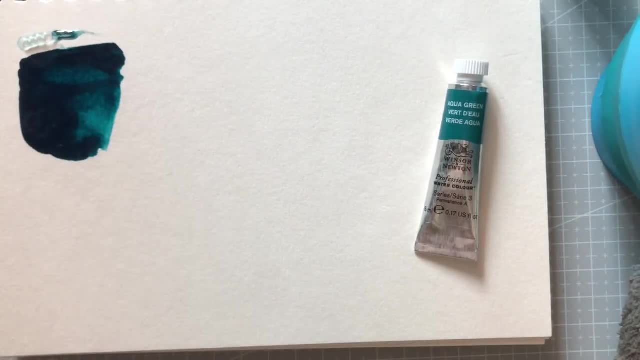 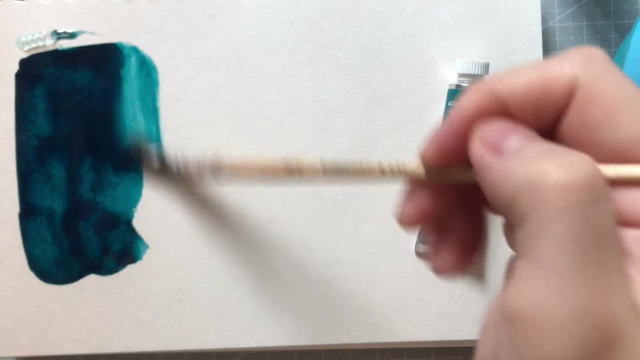 strong tinting, high tinting color, because I believe it is a phthalo pigment. but Winsor & Newton doesn't say whether or like what pigment it is, They just say it's a phthalo pigment. I'll show you on the tube in a bit, but like, look at this. 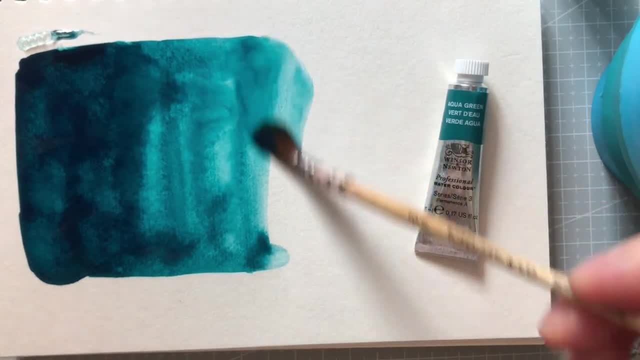 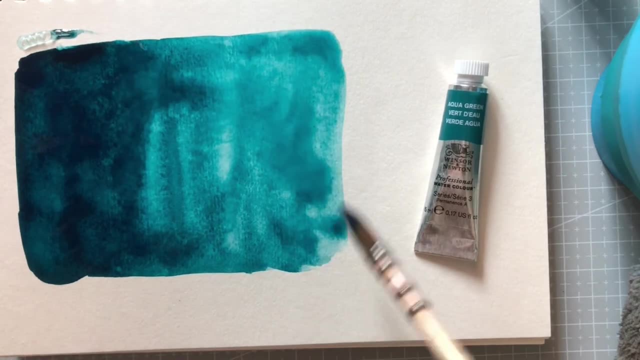 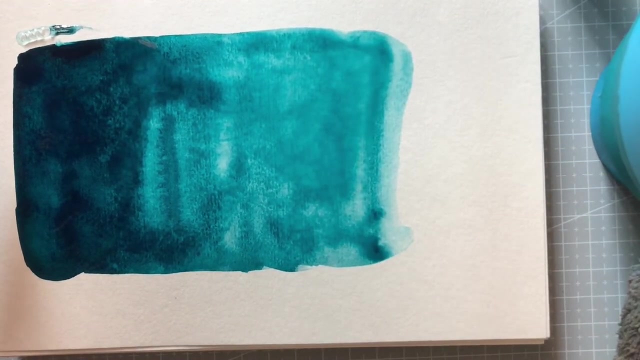 color I would say it leans very green. so for those of you who don't like turquoise but love green, you might want to try this one to get yourself like into turquoise, if that's what you're after. I'm trying to dilute this as much as possible so you could see the color. 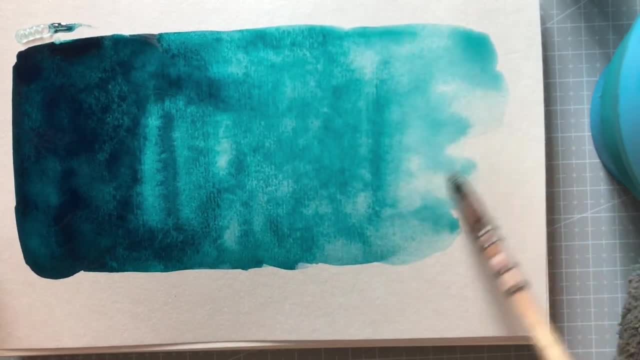 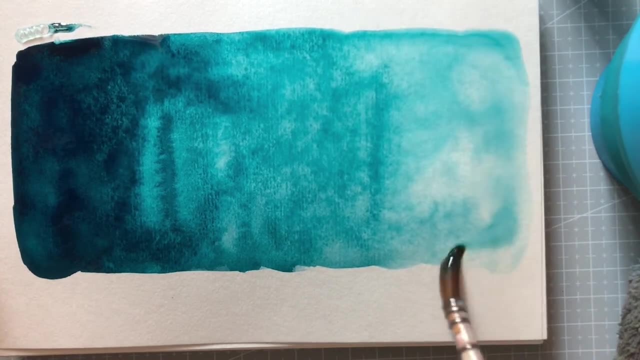 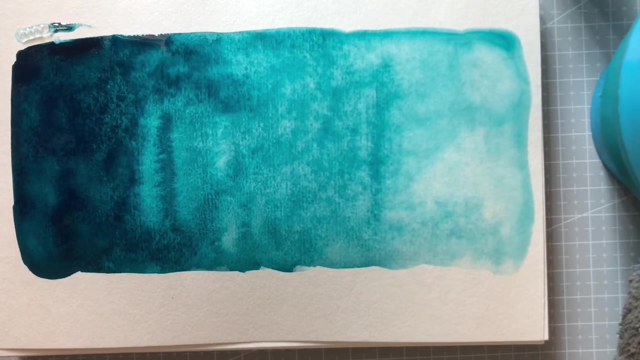 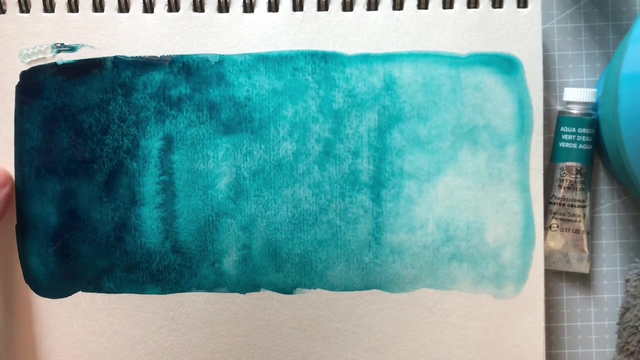 Apparently this one granulates And I am seeing a bit of granulation, but, like, not as apparent as some other granulating colors, And that is what you get Now on screen here. oh no, I'm sorry, the camera's shaking, So on screen here you can see that it's a very dark, dark color in mass tone. It's pretty much. 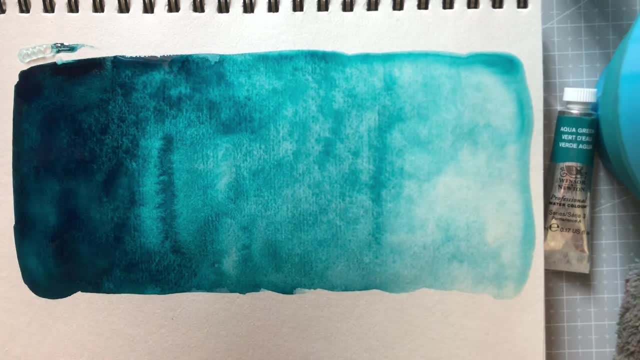 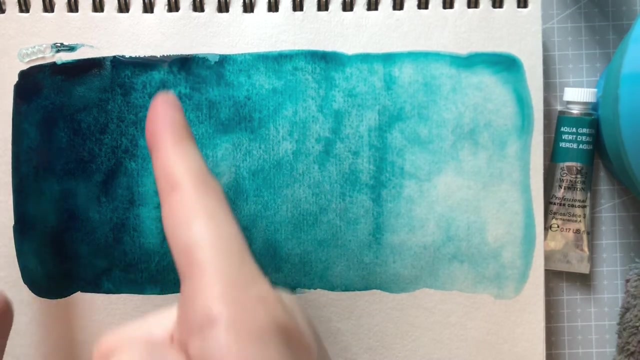 almost black here when it's really pigmented, and then once you get around to like the mid-tones here, you get this like nice, almost, I would say like foresty green, but a cool forest, you know. And if I'm looking at just this section here, it looks almost like Rembrandt's or Van Gogh's dusk. 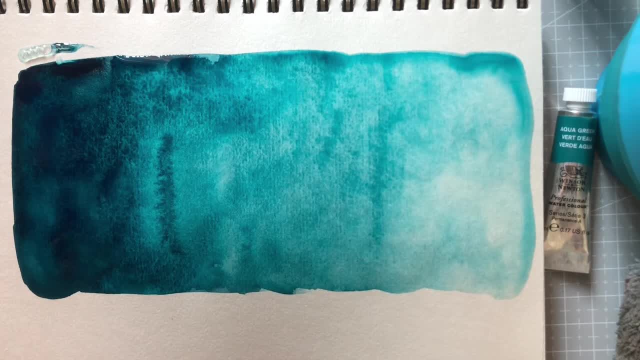 green, where you have like a phthalo green color mixed with PBK 11 or like oxide black, because you get that granulation in there. that's just so beautiful And once you get down here, once it's like more diluted it, it does feel more like a cobalt turquoise because it's granulating. 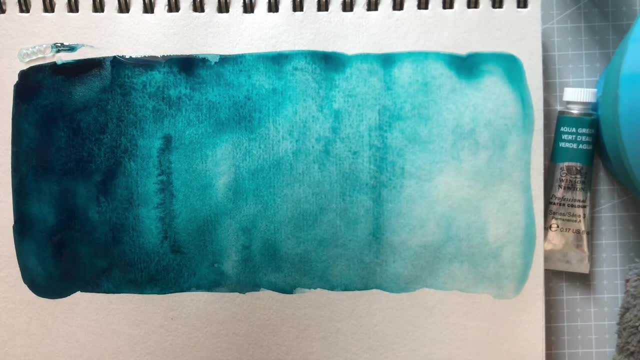 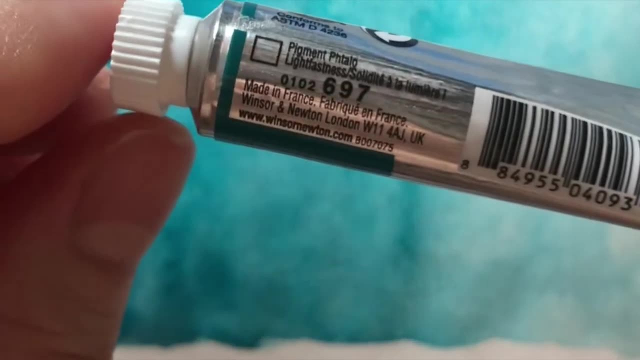 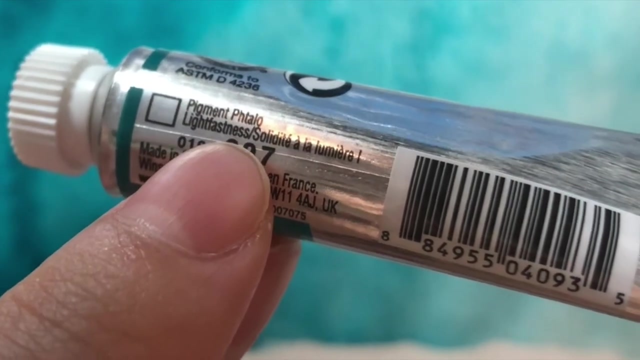 but like a greener cobalt turquoise, or maybe even like cobalt green made with pb26. oh yes, so i should show you. so on the tube and on the website it says pigment phthalo, so there's no pigment number. interesting, why did they spell that wrong p-h-t-a-l-o. 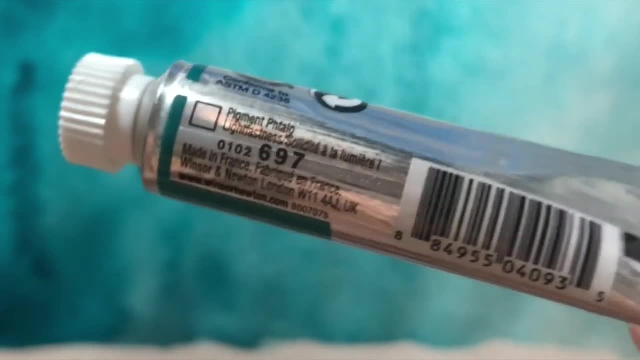 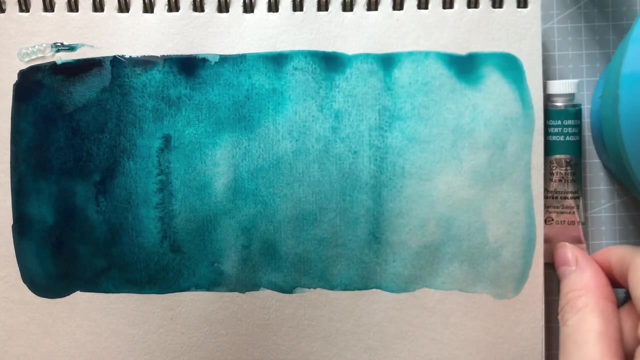 is it supposed to be p-h-t-h-a-l-o? okay, who cares? whatever, maybe it's in a different language anyways. so yes, it's supposedly phthalo pigment, but there's no number. um, i don't know if they're going to assign a number, or maybe they did a mixture of pigments. i don't know. 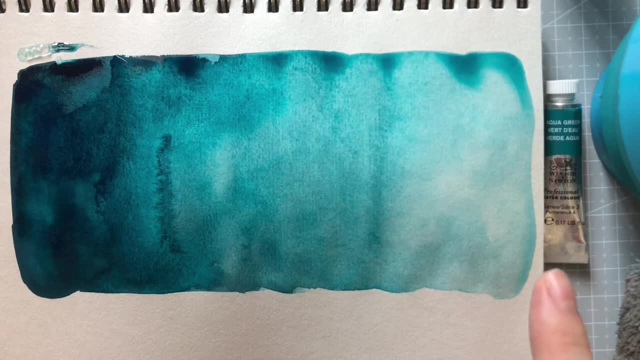 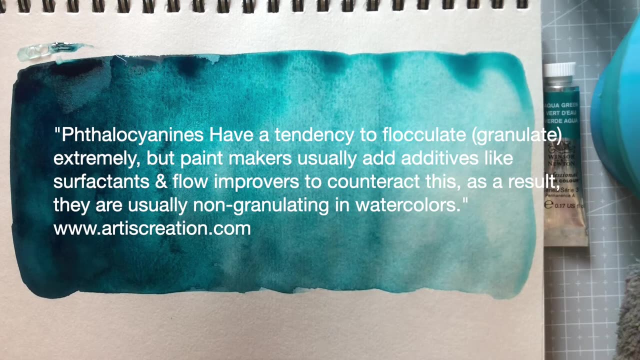 so it's just another hint to say that i don't know, but i would like to note this. interestingly enough, phthalo colors, your phthalo blue. they look greens and all that. they're actually naturally granulating, but when manufacturers make them into paints, somehow they've made it so that it's 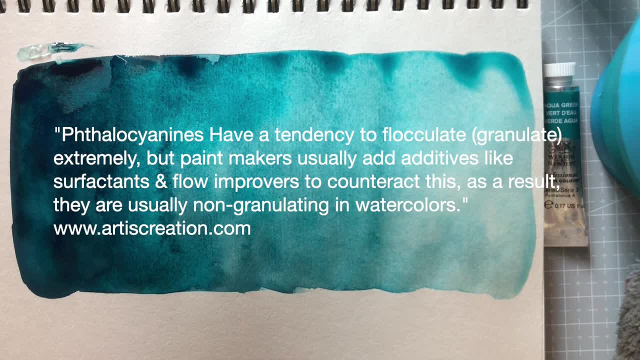 non-granulating, and i wonder why we don't have more granulating phthalos. shouldn't that be something that we're given the choice of? i'm going to put on screen here where i got that information: some more deep research, if you want to. So, before we go any further, I think I'm going to wait for. 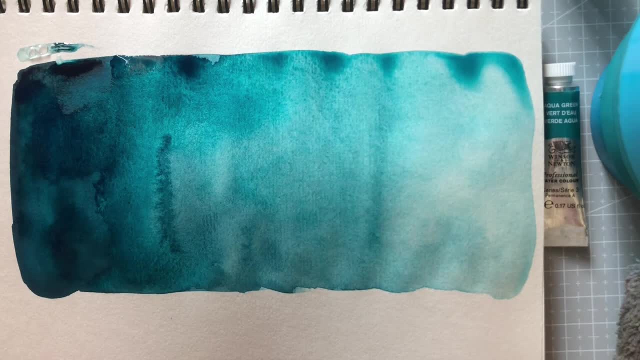 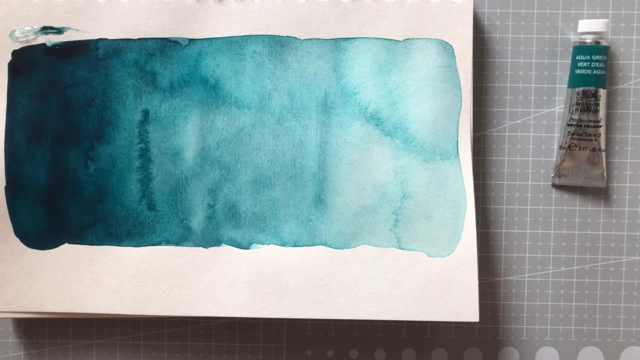 this to completely dry and then come back to compare this with some phthalo turquoises that I've already swatched out. All right, I'm back with the completely dried swatch. As you can see, beautiful granulation. I wouldn't say there's like so much granulation, like your typical. 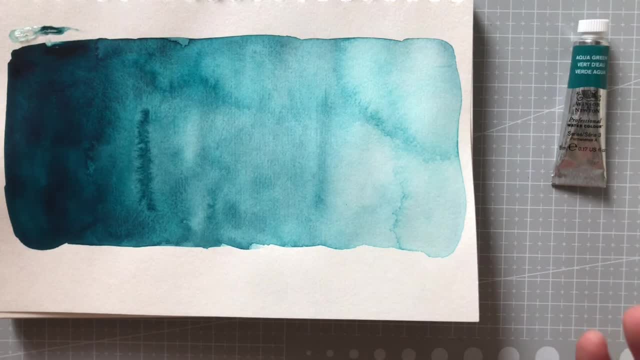 ultramarine blues, but the granulation is there And I also feel like this part here, like in the mid-tones, that's where you get most of the granulation effect happening, And it's also a color that could get really dark, like almost black, once you like layer it or lay down a lot. 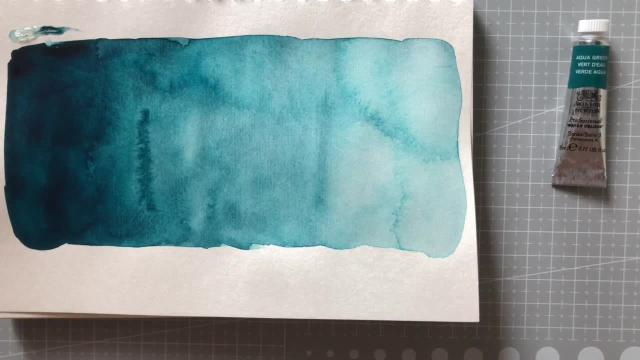 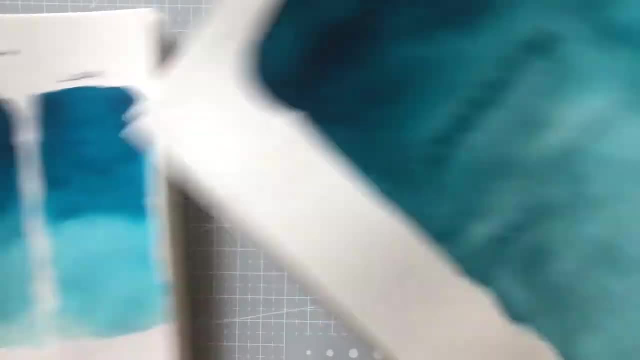 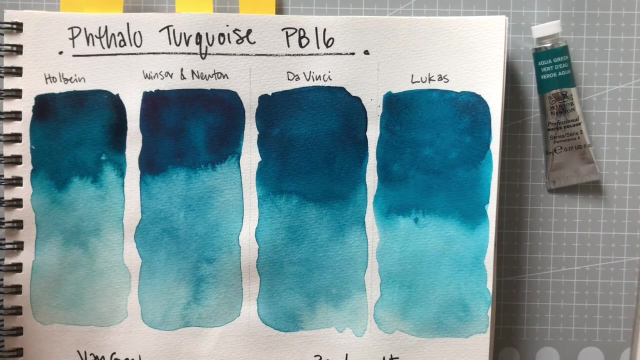 of pigment And for today I particularly wanted to show you it, this aqua green by Winsor & Newton compared to some phthalo turquoises. So if you haven't seen already, I have posted a phthalo turquoise- PB16 comparison video. I'll 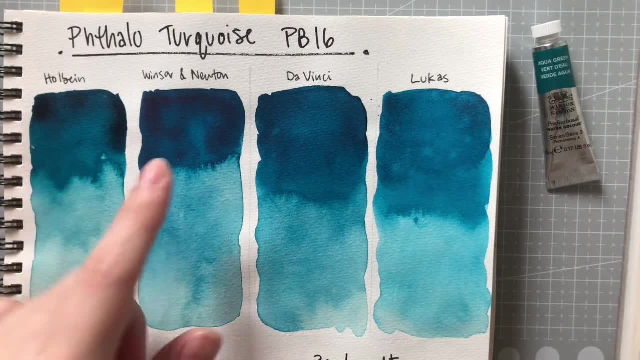 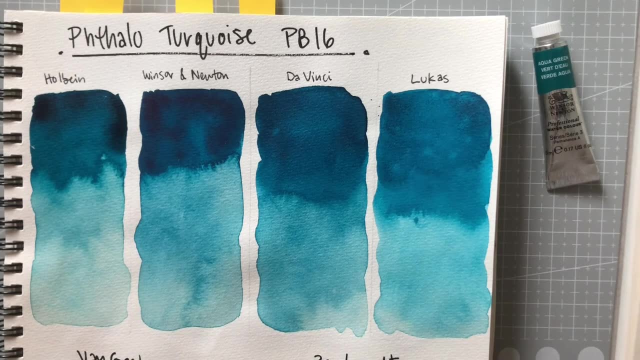 link that down below. So right here I have Holbein's, Winsor & Newton's, Da Vinci's and Lucas's, And since then I've actually received Daniel Smith's phthalo turquoise PB16 from Lark as well. Thank you so much, Lark, And while it's not in here, I can tell you that it's very much. 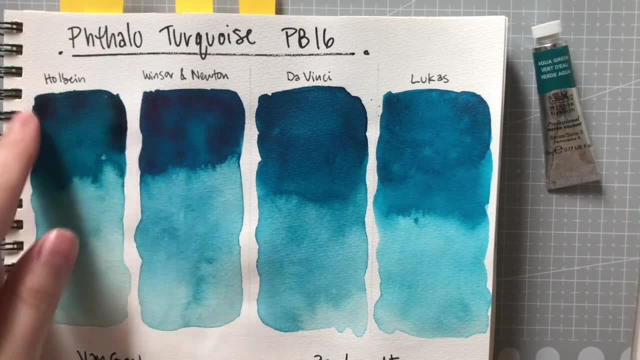 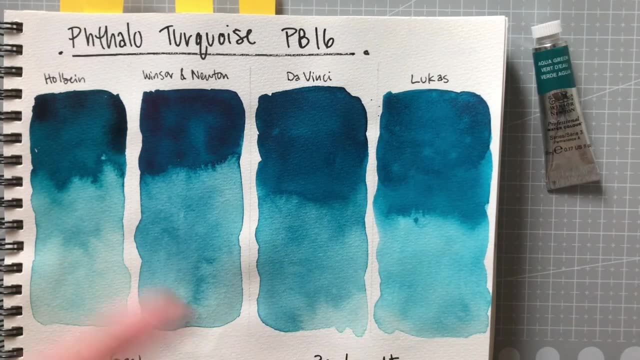 like Da Vinci's in that it doesn't get as dark as Holbein's and Winsor & Newton's, but it is highly pigmented And it's- yeah, it's- basically like Da Vinci's in hue as well. So if we compare aqua green to phthalo turquoise, I'm not sure if you could see it. 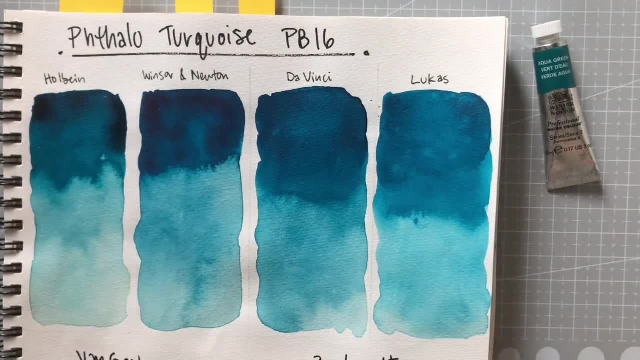 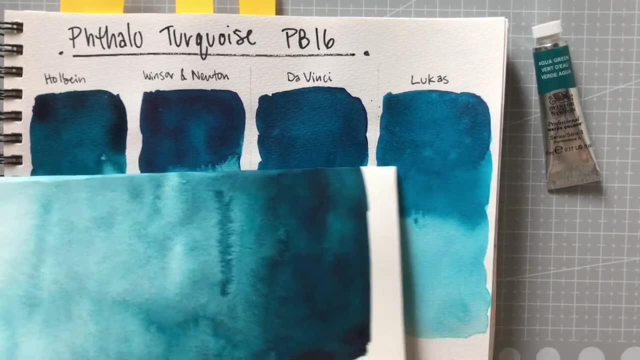 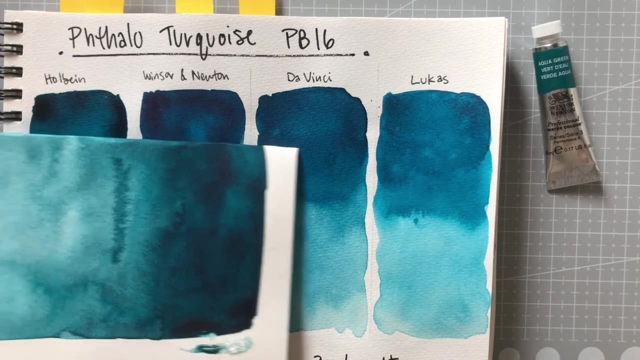 completely. Let me try to. Okay, so I've folded the paper so hopefully you could compare it. You could see the comparison, but basically. Okay, so I'm looking at the viewfinder here and it's not very clear. 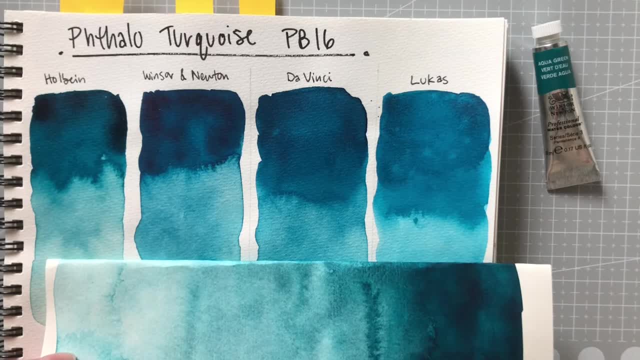 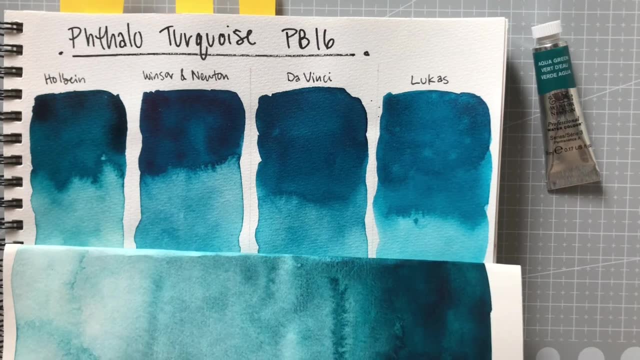 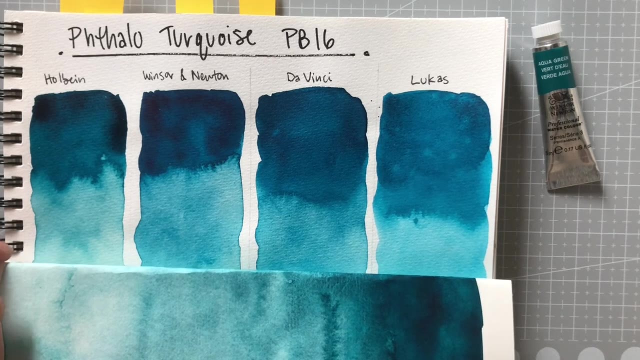 It looks pretty identical on the viewfinder, but I guess I'll have to tell you myself. then. I'd say the hue of aqua green is cooler than the phthalo turquoises you see here. By cooler I mean it's greener. So Holbein's is the greenest of the bunch here that you see today. 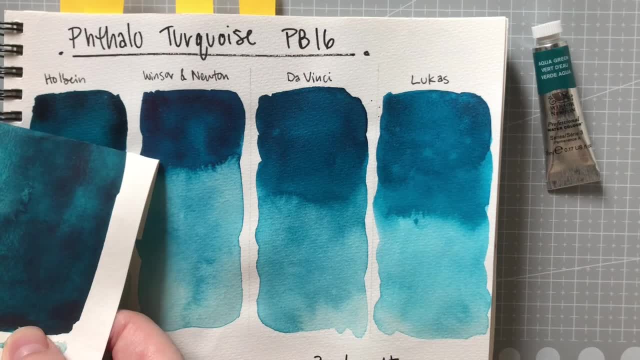 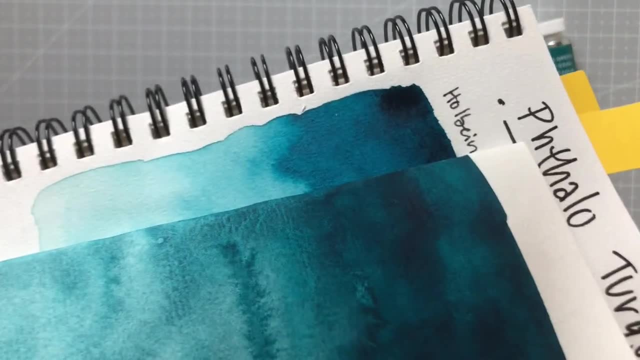 And Winsor & Newton's aqua green is the slightest bit greener than Holbein's. So that's Holbein's up there And then if I do, If I do this, hopefully you can see that Winsor & Newton's aqua green is the slightest bit greener.